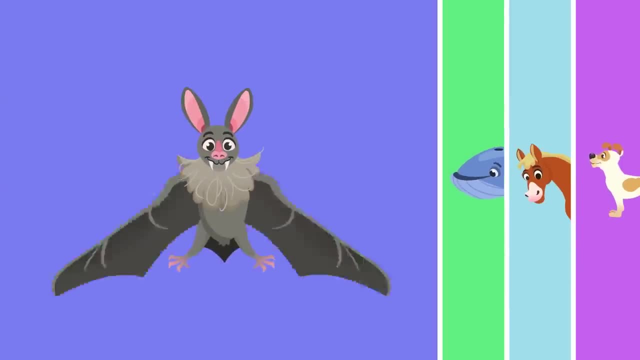 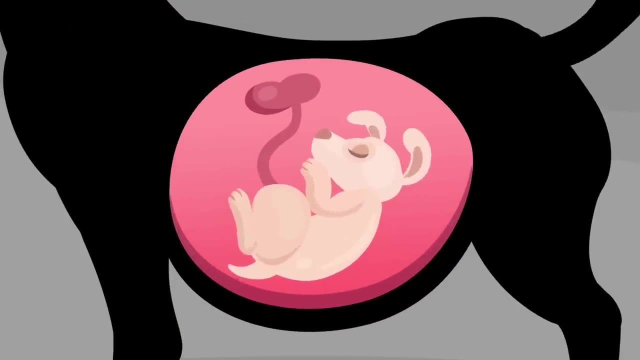 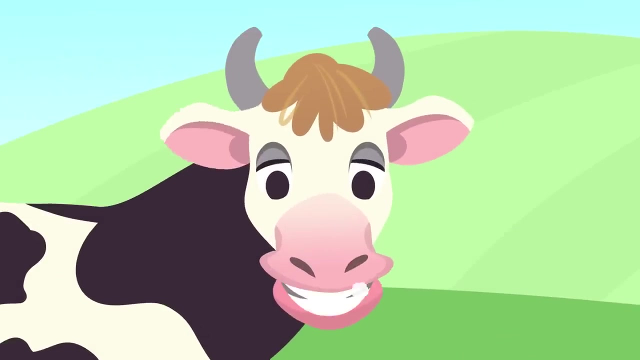 Do you know what kind of animals these are? No, That's what I'm here for. Mammals are viviparous animals, meaning they are born from their mother's womb. Mothers have mammary glands that give milk to feed their young Inside their mouth. they 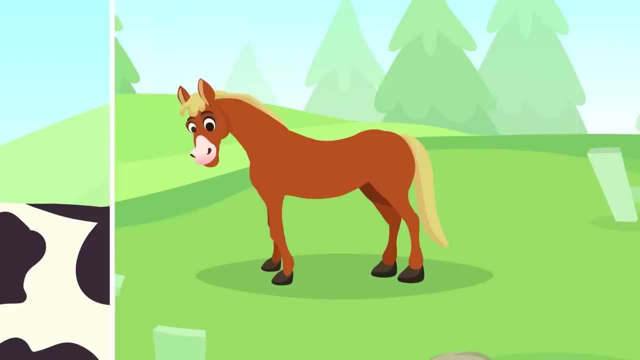 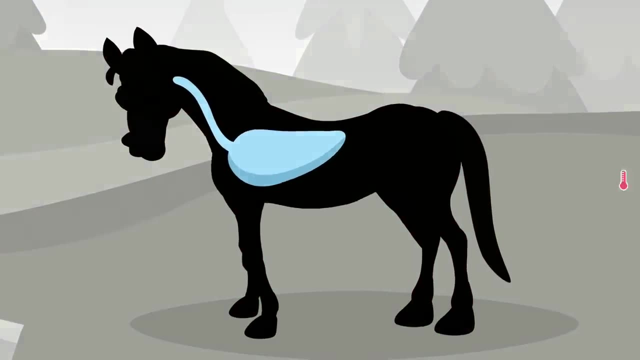 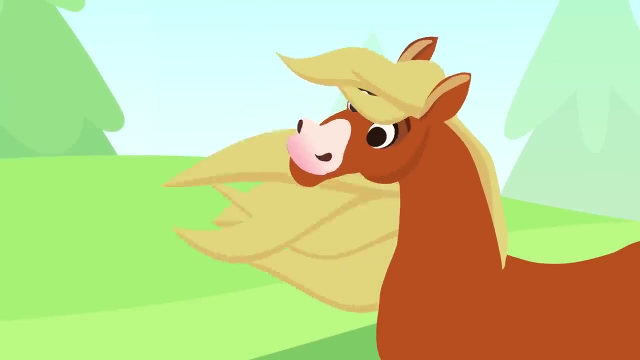 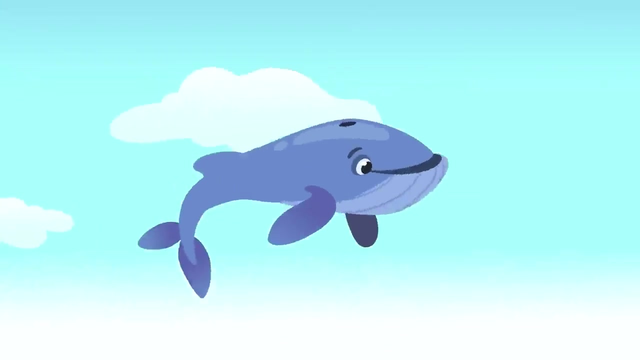 have teeth to chew their food. Mammals breathe through their lungs. They are warm-blooded animals- warm-blooded animals, and the majority of them have hair covering their bodies. They can live on land, in the water, and some can even fly. 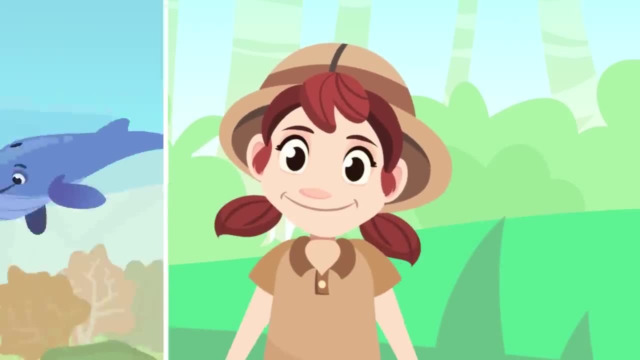 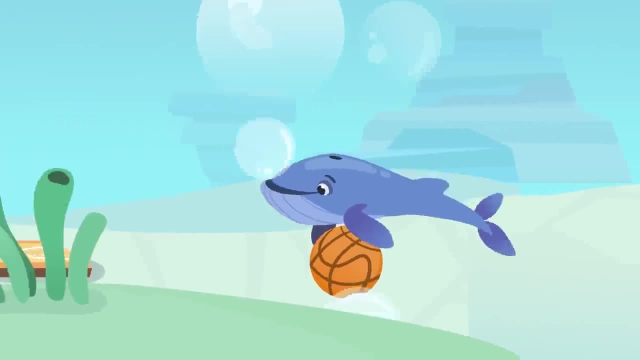 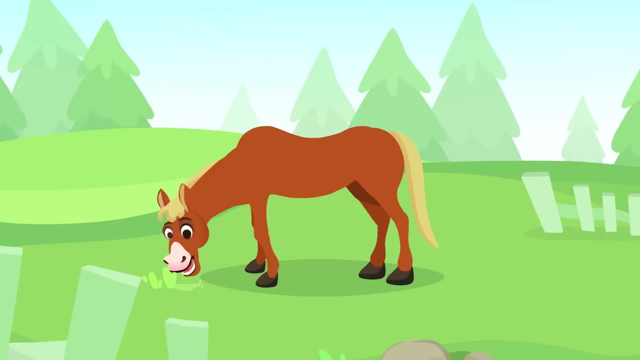 And now some fun facts about mammals. The biggest mammal is the blue whale. It can measure up to 30 meters long, a little more than a basketball court. Oh, A horse is another mammal. Did you know that its teeth don't stop growing? 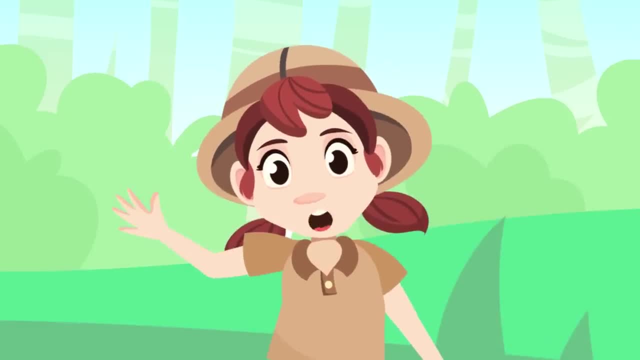 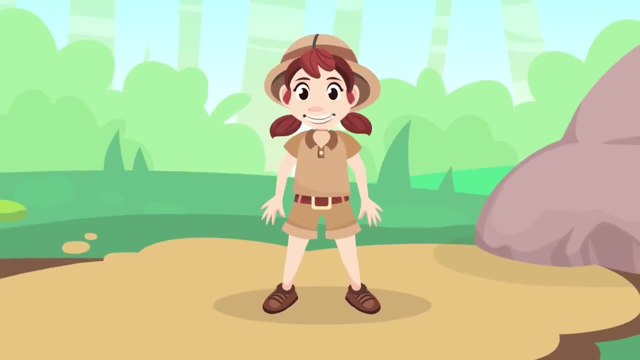 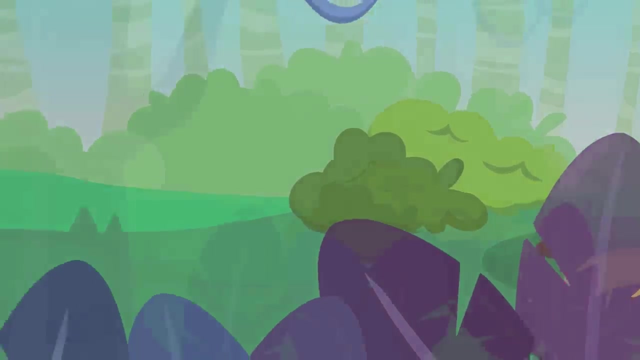 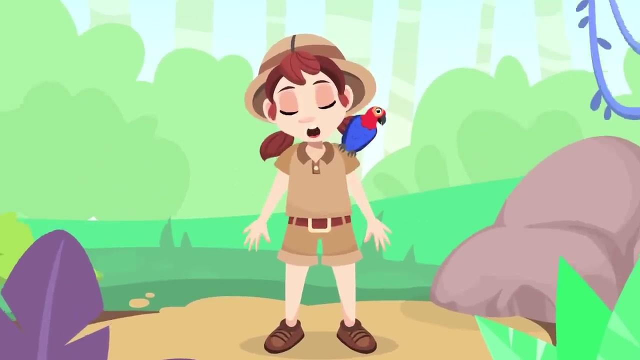 throughout its whole life. And here you have another mammal. What? Where is it? It's me. We humans are also mammals. Well, I am going to keep practicing my dance. See you later. Hey guys, Are you ready to learn a few things about animals? 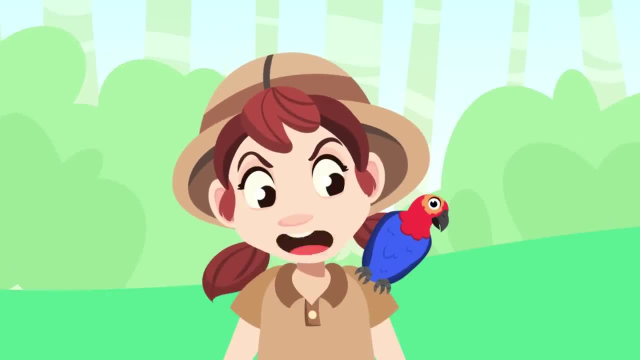 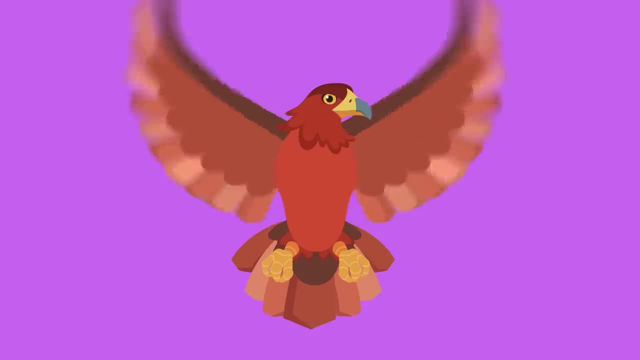 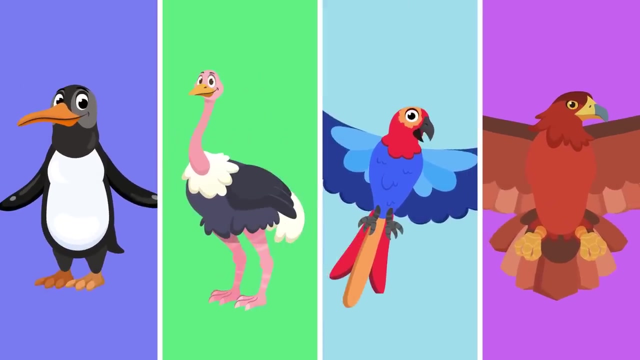 Animals, Animals. Hey, don't repeat what I say. Same, Same, Oh, always the same. Well, guys, today we are going to talk about another group of vertebrate animals: birds, Birds, Birds, Birds are oviparous animals which 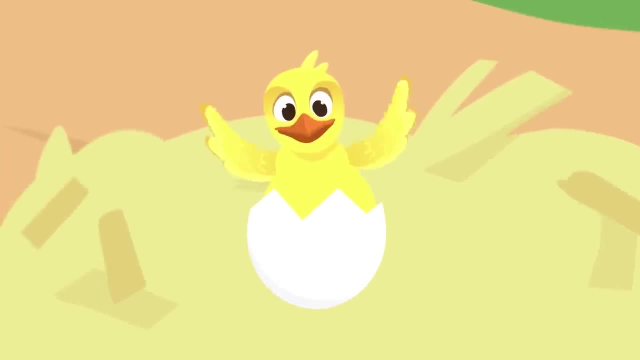 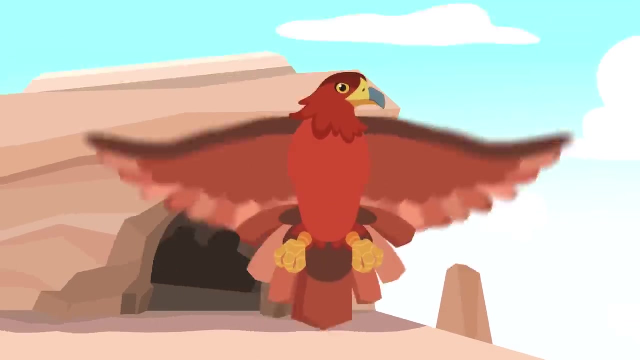 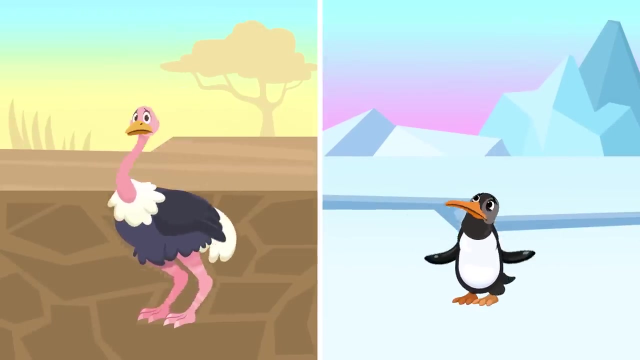 means they are born from eggs. Oh, They have two legs, They walk with two legs And they have two wings that allow them to fly, Although there are some birds, like the ostrich and penguin, that don't fly even though they have wings. 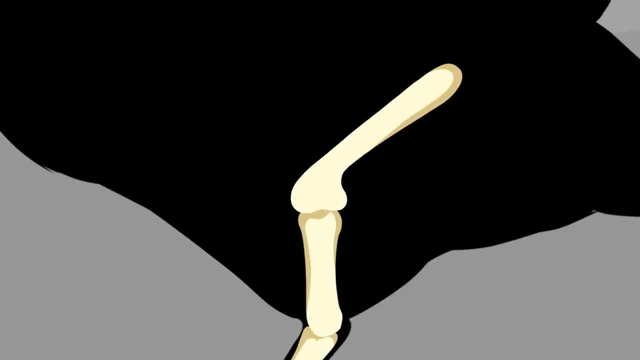 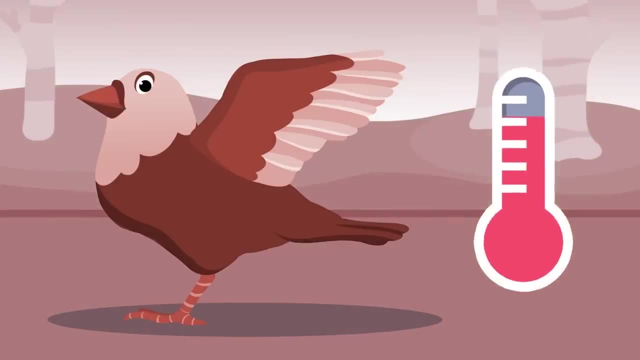 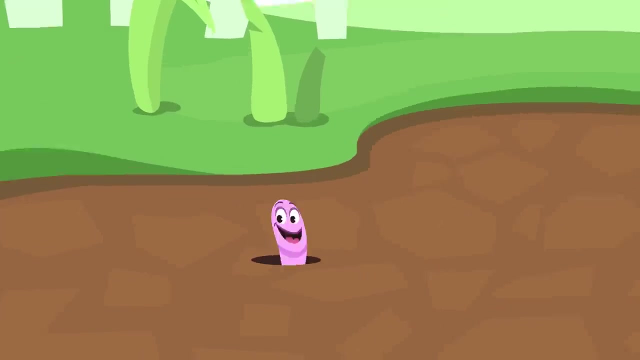 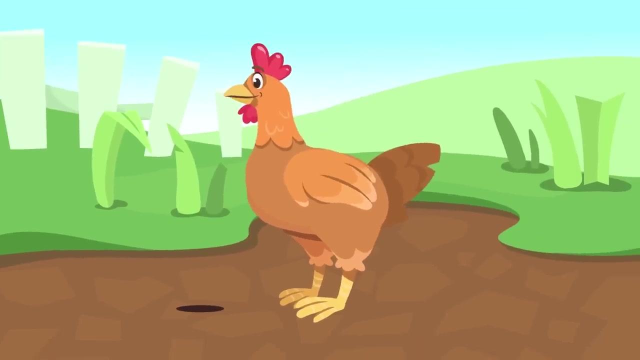 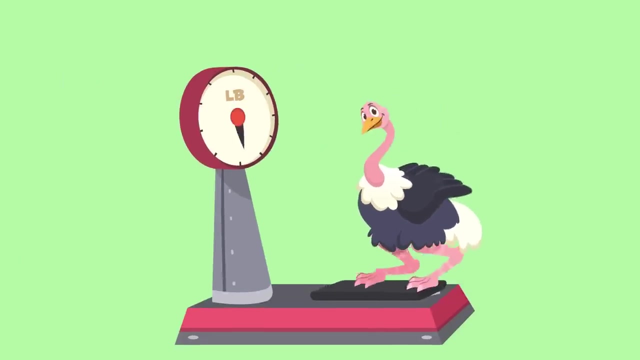 The bird's skeleton is light because their bones are hollow. Birds can breathe thanks to their lungs- their lungs- And they are warm-blooded. They eat with their beak that has no teeth. Their body is covered in feathers. Did you know that the heaviest bird in the world is the? 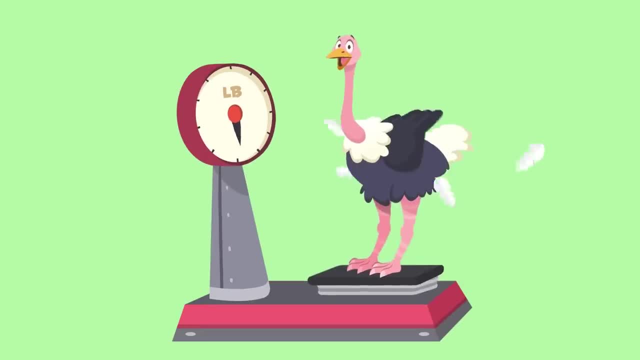 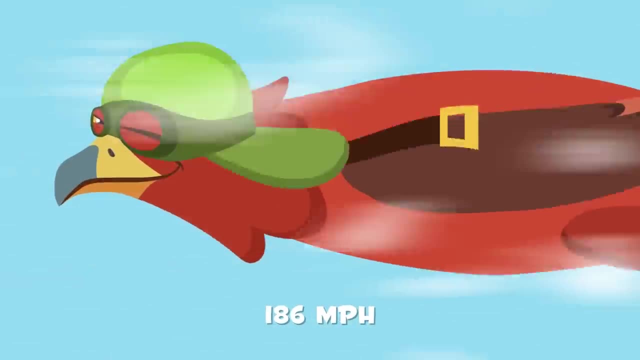 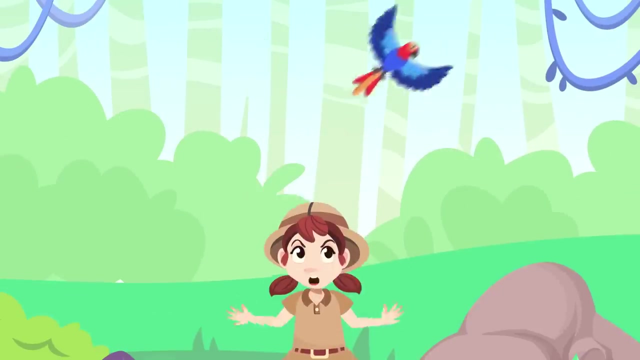 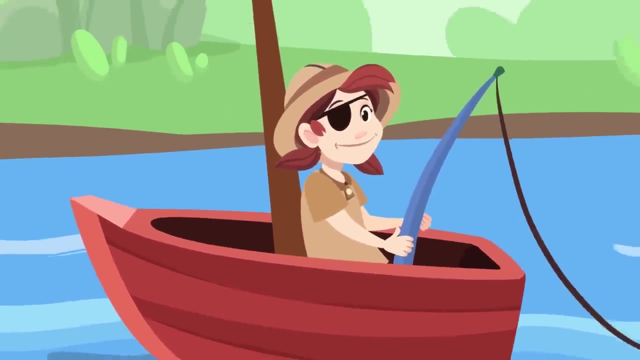 ostrich. No wonder it can't fly, Poor thing. A bird that can fly is the eagle. Incredible, Incredible, Incredible. You again, Watch what happens if I catch you. Hello, Hello, How are you mateys? Not one is biting. Well, later I will continue because 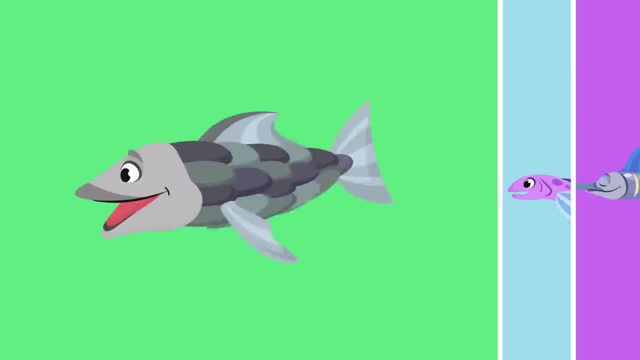 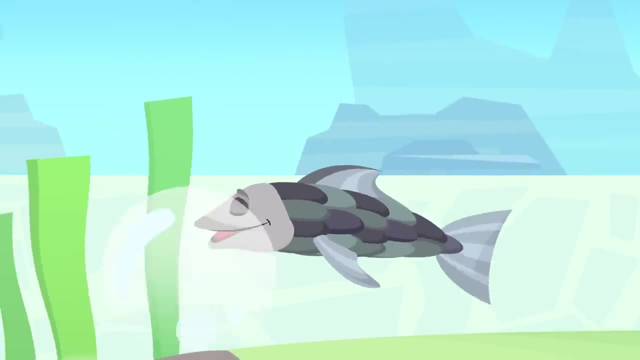 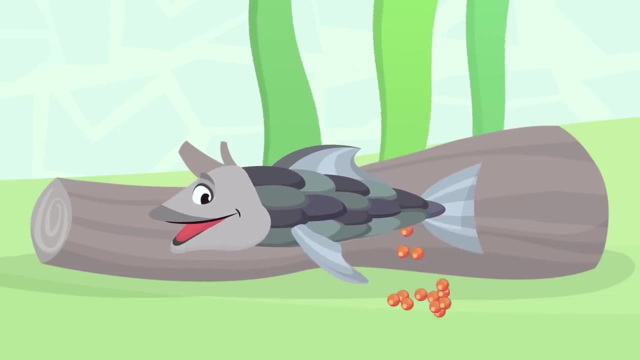 two of them are biting. Today I am going to talk to you about another group of vertebrate animals: fish. Fish are aquatic animals that can live in freshwater or saltwater. They are oviparous, meaning they are born from eggs, They have fins to move around the water and they have a tail. 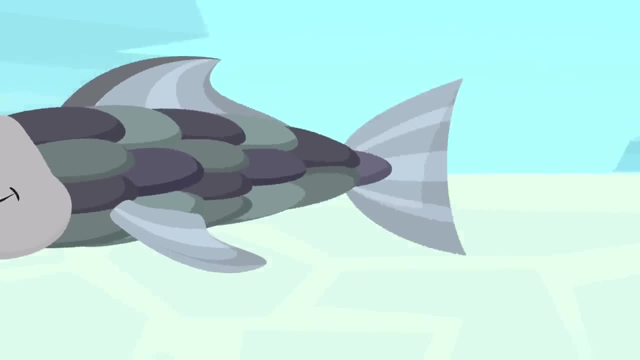 at the end of their bodies, helping them to swim easily. As you can see, their bodies are covered in scales. They have a tail at the end of their bodies, helping them to swim easily. As you can see, their bodies are covered in scales. They have fins to move around the. water and they have a tail at the end of their bodies, helping them to swim easily. As you can see, their bodies are covered in scales, They have fins to move around the water and they have a tail at the end of their bodies, helping them to swim easily. 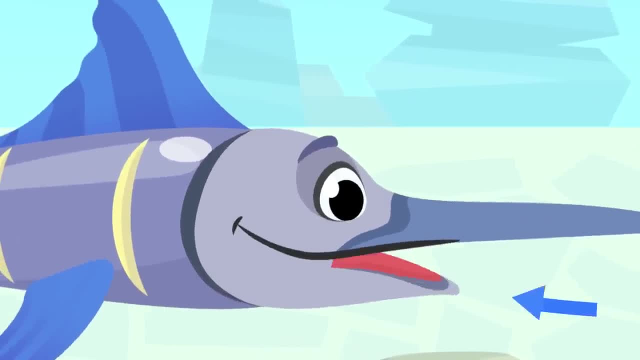 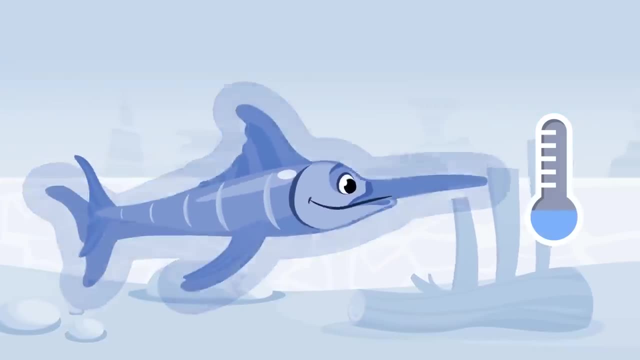 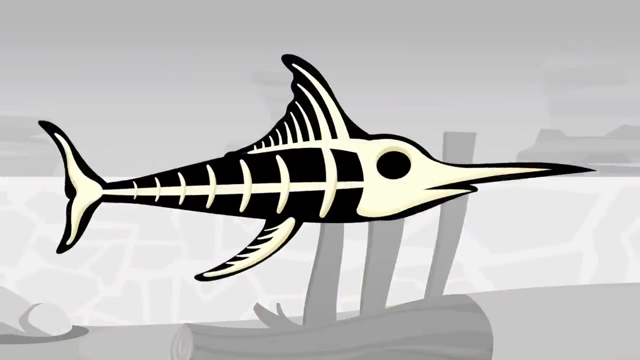 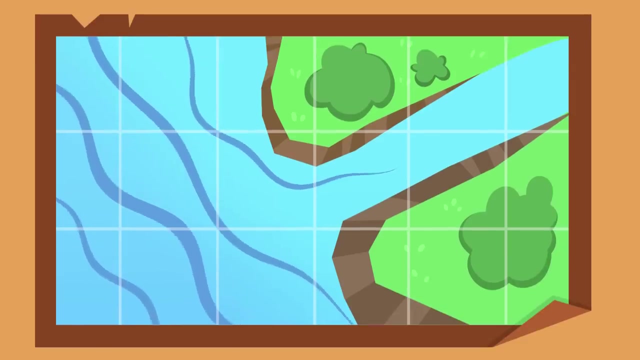 Because they are aquatic animals, they breathe through their gills. They are cold-blooded animals, which means their body temperature varies depending on the water temperature, And they have a simpler skeleton than other vertebrates. Did you know that there are fish like salmon and eel that travel all the way? 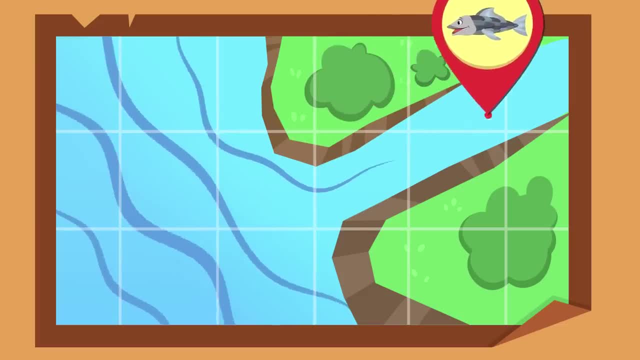 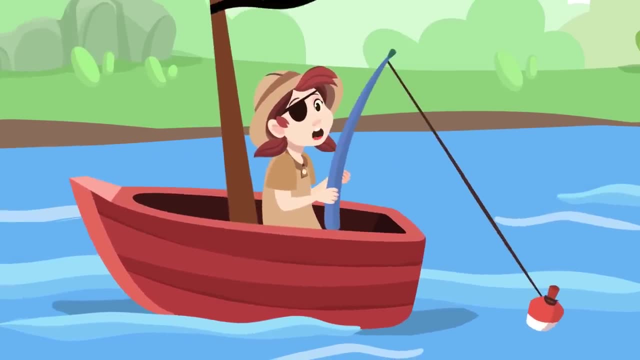 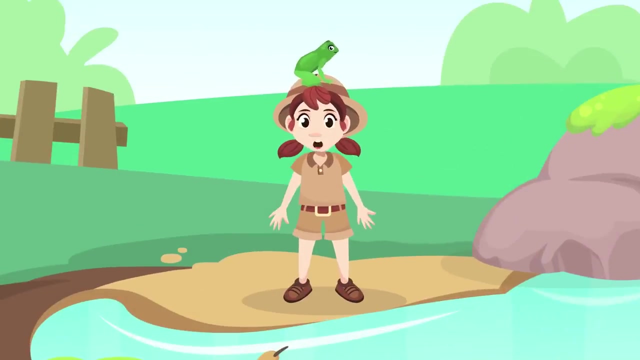 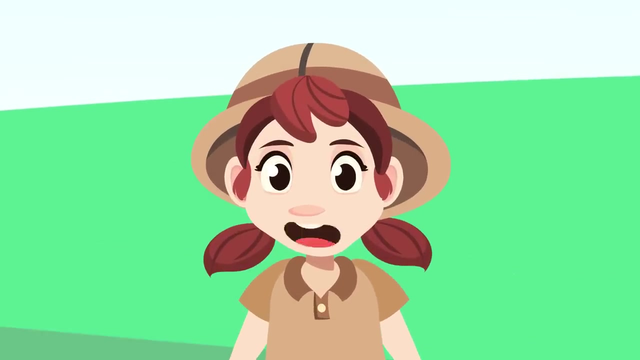 From areas of salt water to areas of fresh water. What a trip. And that is all about fish. Oh, I think I've got something. See you later. How's it going, guys? Today we are going to talk about: Oh, I had a frog on my head and you didn't even tell me That was scary. 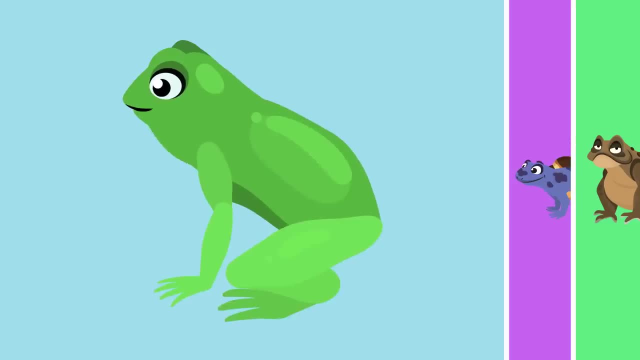 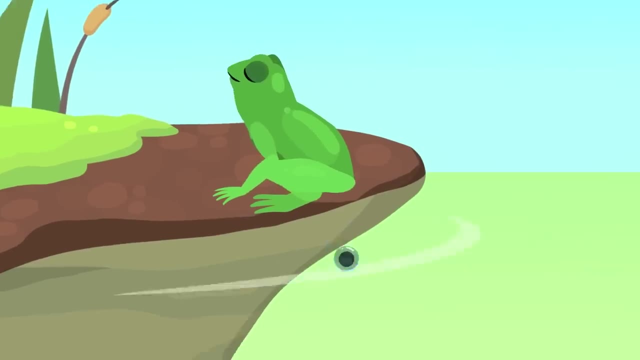 Well, today I have come to talk to you guys about another group of fish that are very likely to do better than other vertebrates, And that group of fish is called amphibians, and they are an amphibian. Amphibians are oviparous animals, which means they are born from eggs. 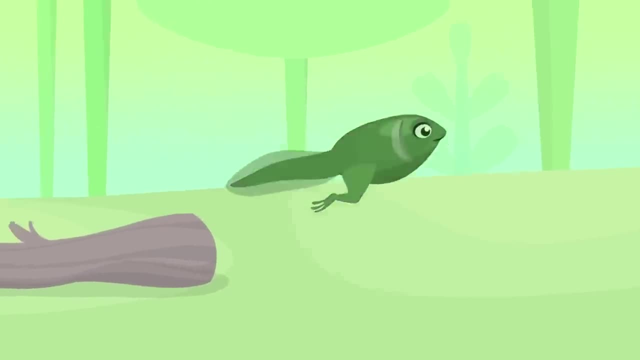 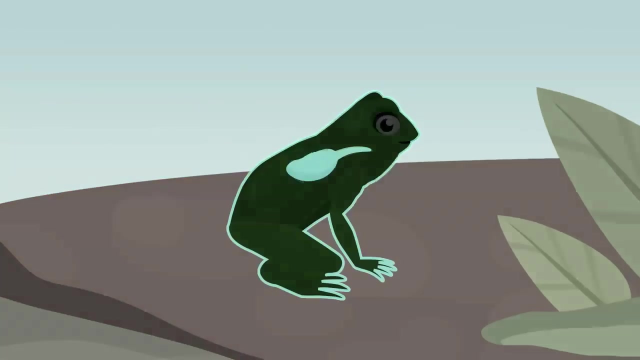 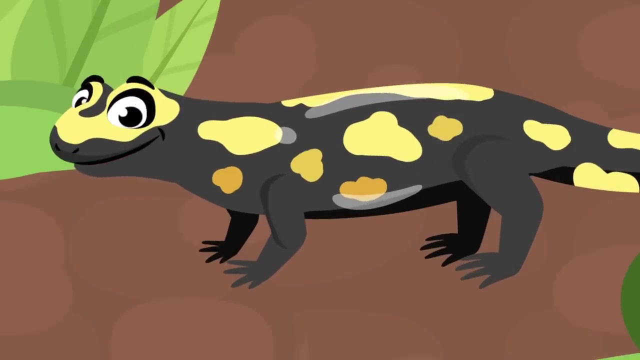 The babies are born in the water and breathe through their gills. When they grow up, they can live on land or in the water and breathe through their lungs and skin. Their skin is moist and they don't need hair. I will show them how to move their body with a frog. 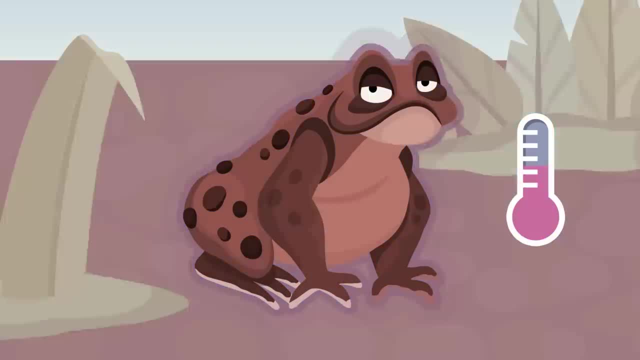 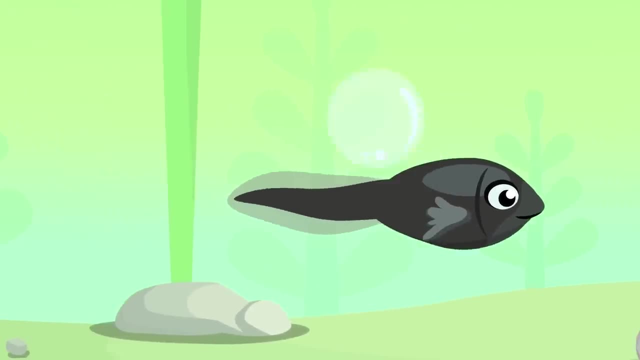 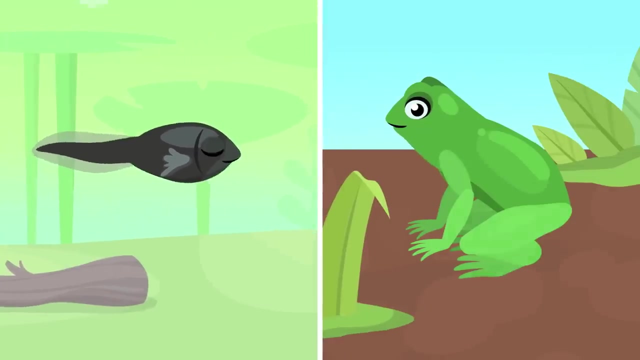 They are cold-blooded animals, which means their body temperature varies depending on the air temperature. Did you know that amphibians are the only vertebrates that are born with a tail and live in the water? When they get bigger, they grow four legs and live on land? 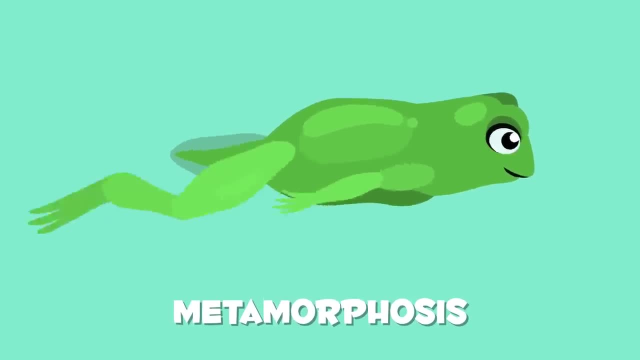 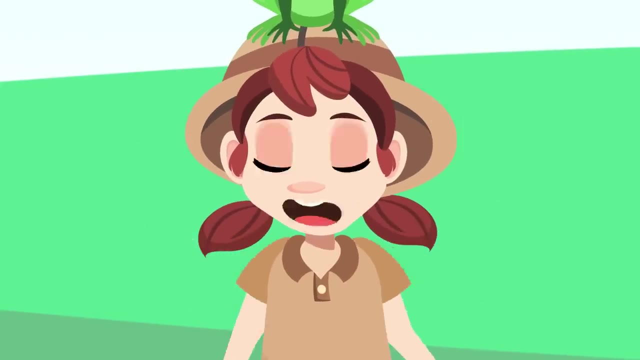 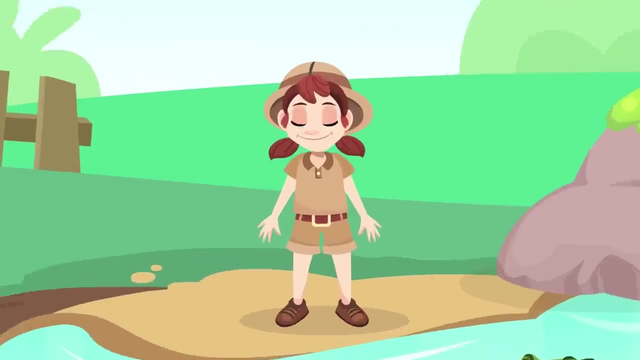 This change is known as metamorphosis. That's everything about amphibians, friends. I hope you guys liked it. I'm going to stay here with my new friend. See you later. Hi, friends, Today we are going to talk about another group of vertebrates. 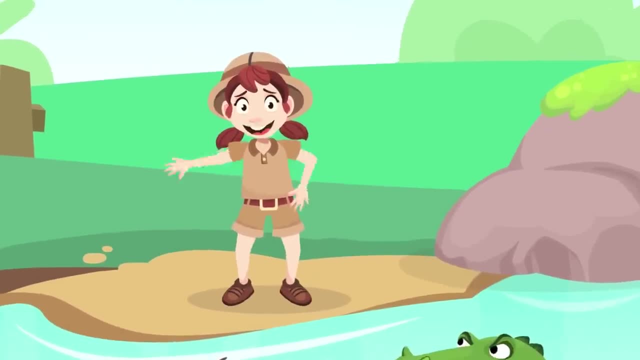 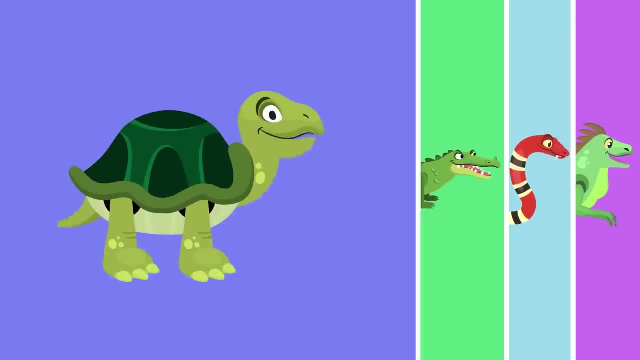 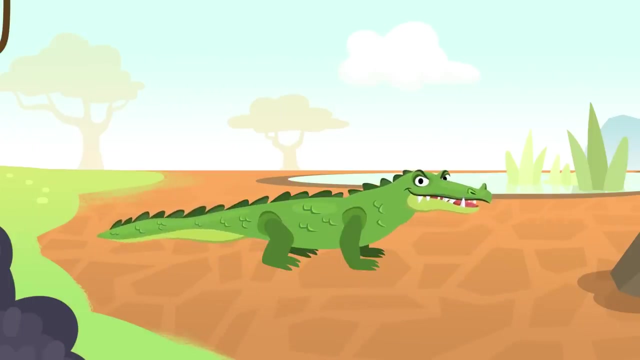 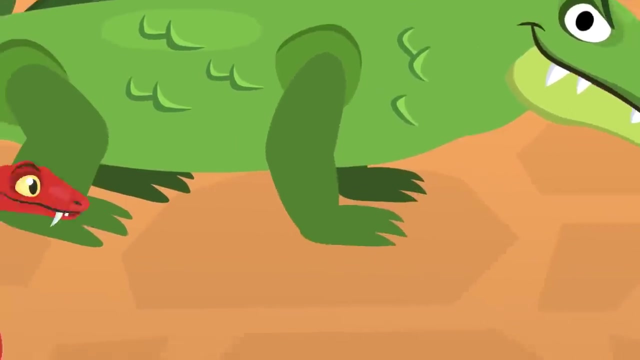 Today we will talk about- Oh, it almost got me. Today we will talk about reptiles. Oh, Reptiles are oviparous animals, meaning they are born from eggs. Their bodies are covered in hard scales. Their legs are really short.